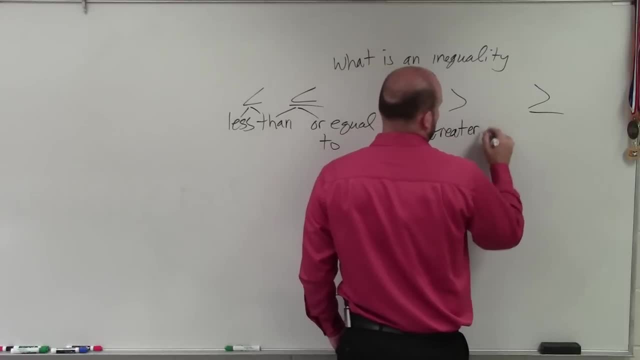 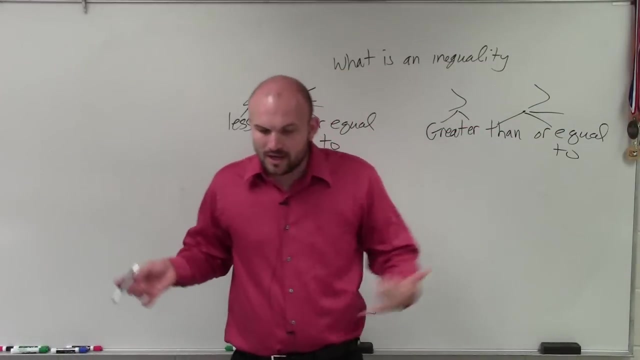 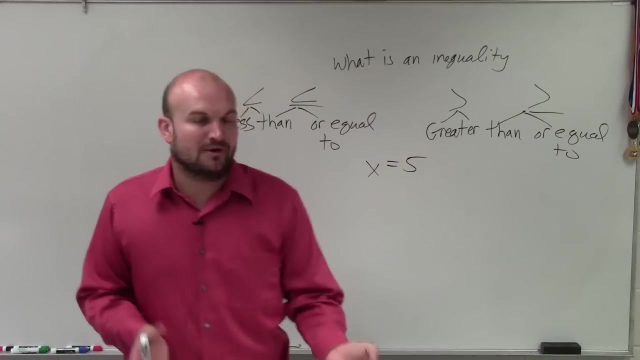 than or equal to. Okay, So pretty much this just says this just represents greater than And this says greater than or equal to. So, looking at an equation, you know, if I give you an equation- x is equal to 5.. Well now, based on that equation, we know that the value of x is the 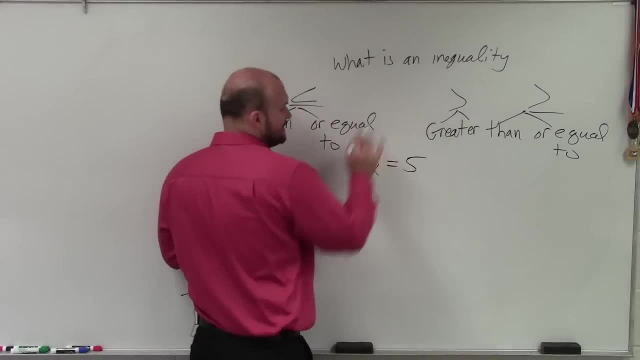 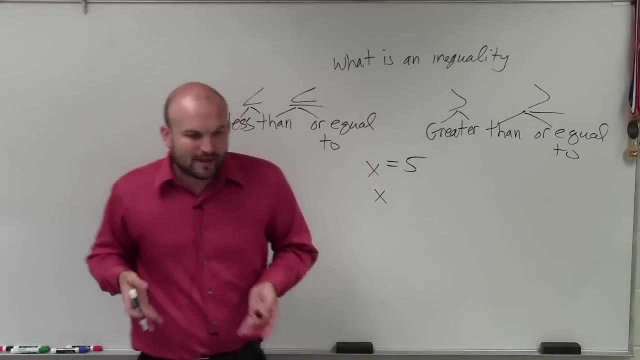 same as 5, right, But when we start using these inequality symbols? So, or anyways, let me go back, kind of go back to the equation again. So therefore, we know that equation is true only when the value of x is equal to 5.. Because, if I plug, 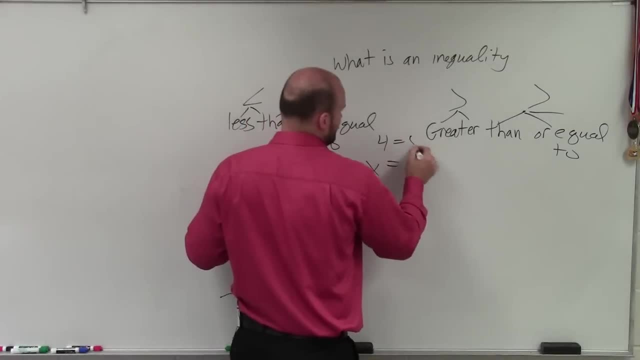 in a value of 4, in for that, you know, 4 equal to 5.. Let's say the value of x is 4.. Well, obviously 4 is not equal to 5, right? Those are not the same values. So therefore that. 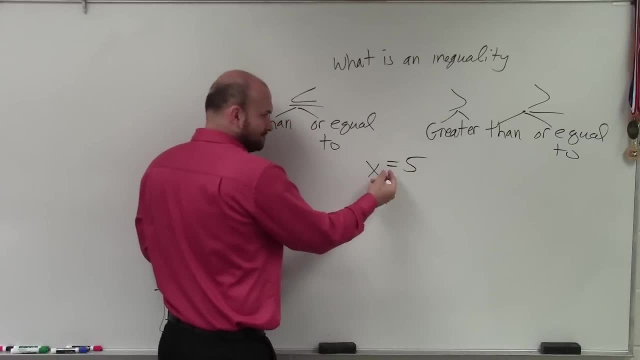 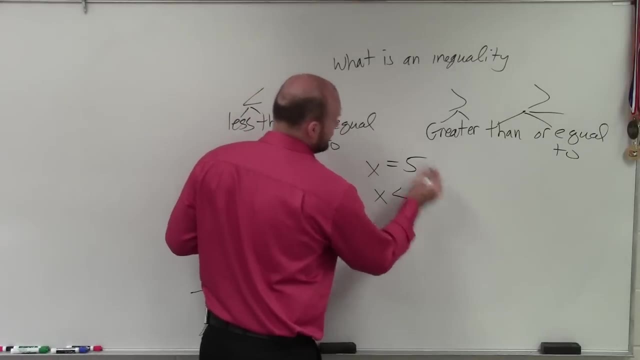 is not equal. So the only time an equation is equal is when, and for this equation is when 5 is equal to 5.. 3.3.. have an inequality. now it's saying x is less than 5.. Well, there's multiple solutions, right? 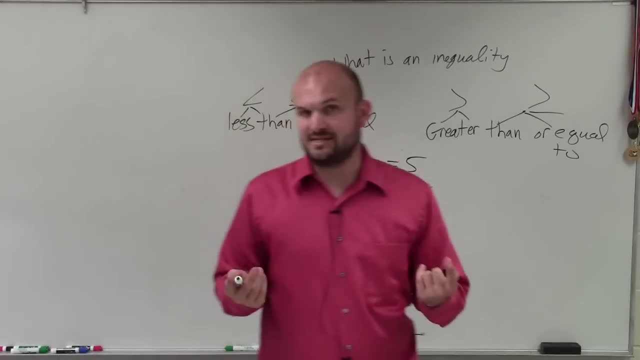 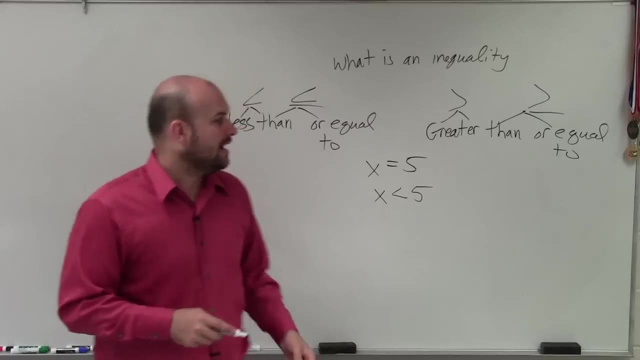 There's going to be multiple answers. You could have negative, Negative. 1 is less than 5.. 2 is less than 5.. 1.7 is less than 5.. 2 thirds is less than 5.. 0 is less than 5.. 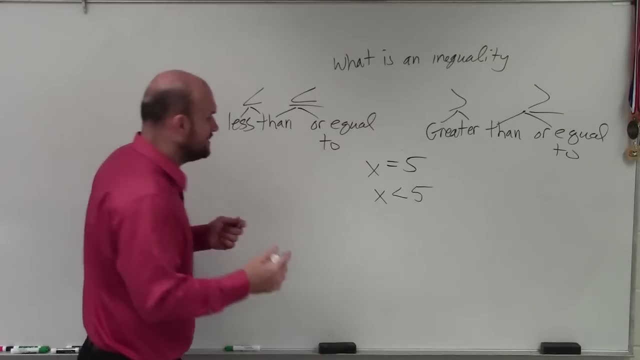 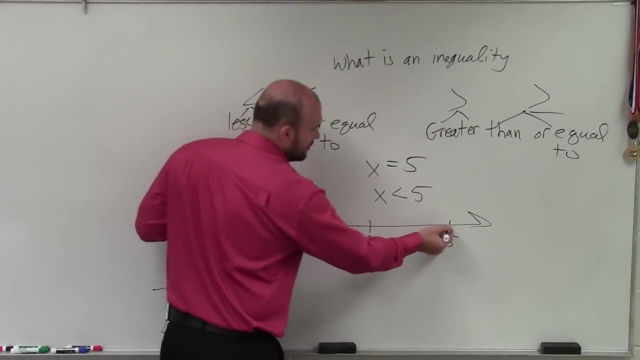 So there's infinite many solutions, And so that's why what we like to do is we like to set a graph, Or, I'm sorry, we graph our solution. So if I say here's 5,, here's 0,, what we do 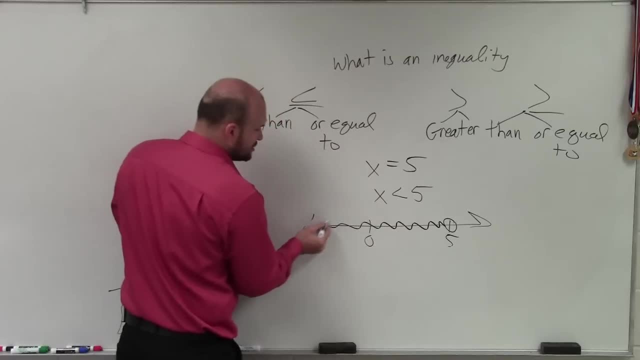 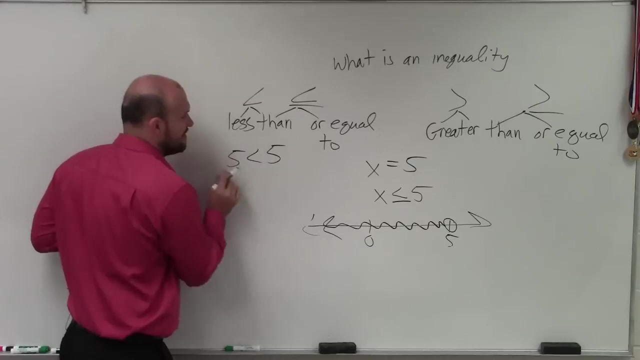 is, we put a circle at that point and then we shade 2.. And this shading represents all the points, that are all the solutions that make this inequality true. The next thing is: what about when I say less than or equal to? Because when I write in, 5 is less than 5, that is false. 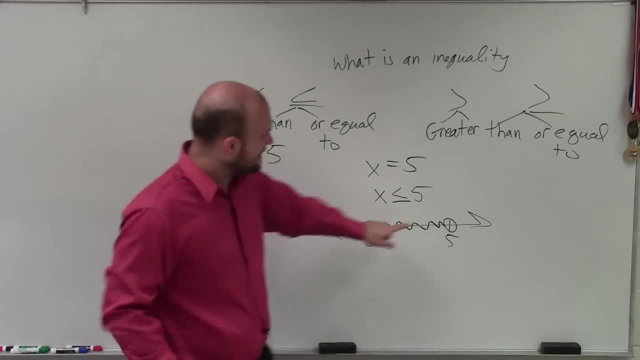 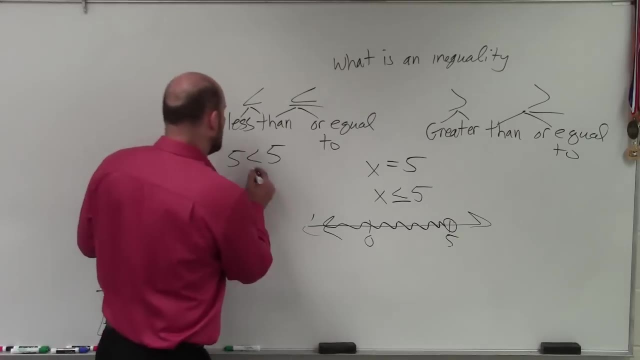 right. 5 is not less than 5, right. So therefore, that's why we leave the circle open, because it's not a part of the solution, But that's still going to be kind of like our starting value, However, when I say 5..